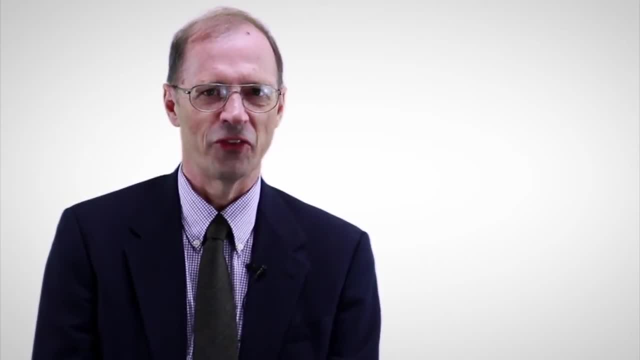 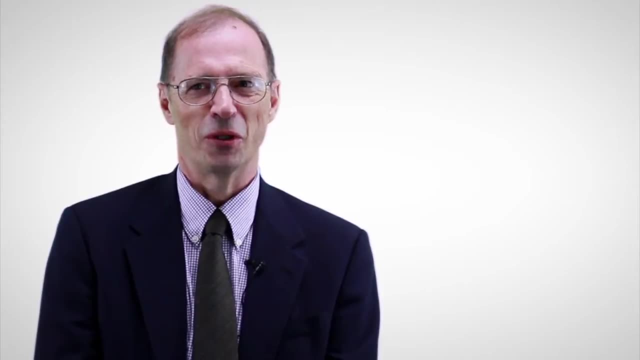 And once in a while I tried experiments. I am known for having caused explosions to occur. None of it ever caused any damage to anybody, I'm happy to announce, But nevertheless that got me interested in chemistry as a career And subsequently when I was thinking about going to college. 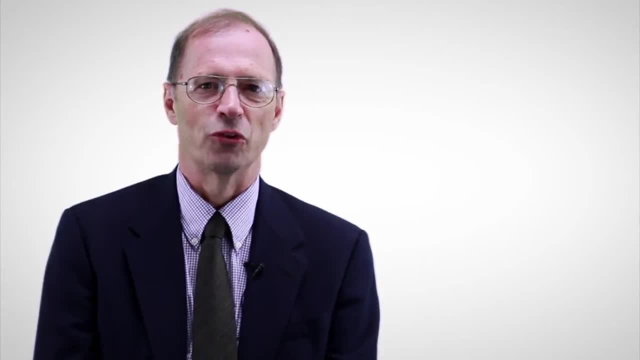 it was a very natural thing for me to think about majoring in chemistry. The good news is that as a college student I had some wonderful professors who got me further inspired about being involved in chemistry. In particular, they got me involved in research programs as an undergraduate student. 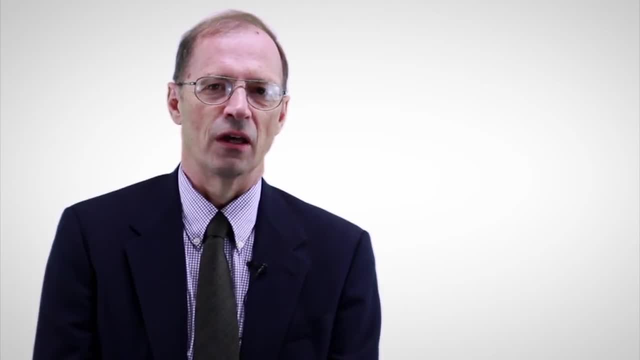 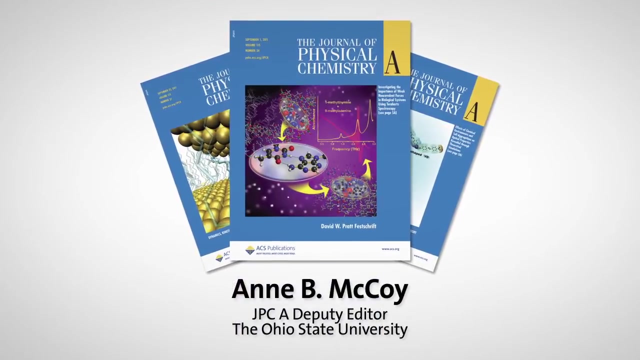 in various types of programs, And this further inspired me to go on, And eventually I went on to get a PhD degree in chemistry And then, from thence, I became a professor of chemistry and that's my career. In the mid-70s we started getting computers into the schools. 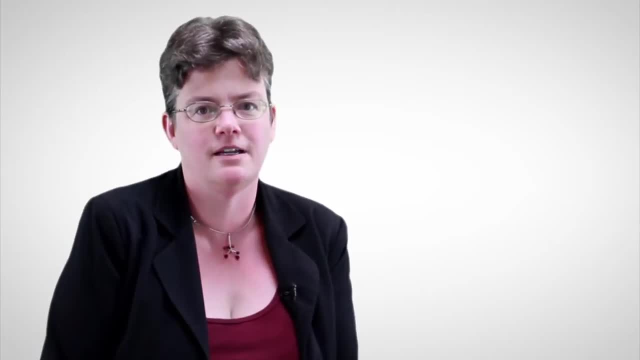 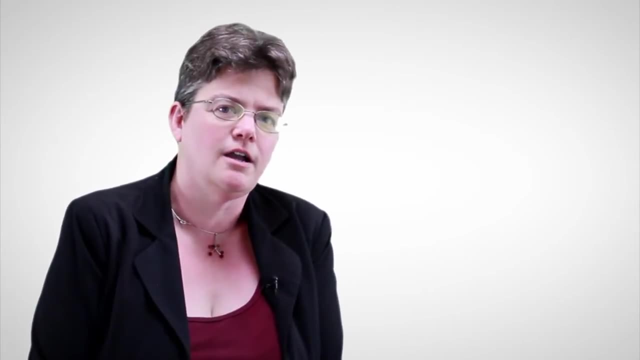 And my mother, who had worked for IBM earlier on, decided that me and my classmates should not just be using these computers for tutorials but should learn how to program. And so I started programming in basic in about the sixth grade, enjoyed the computer part of things, and when I got to high school, 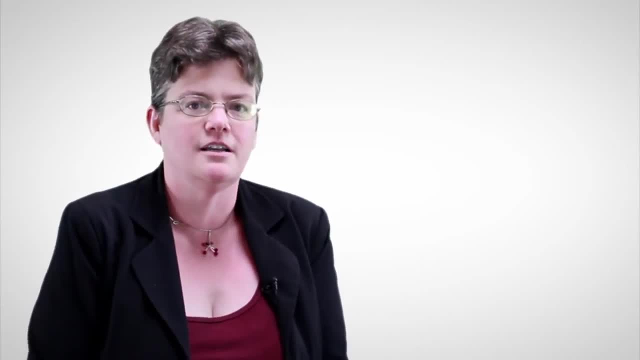 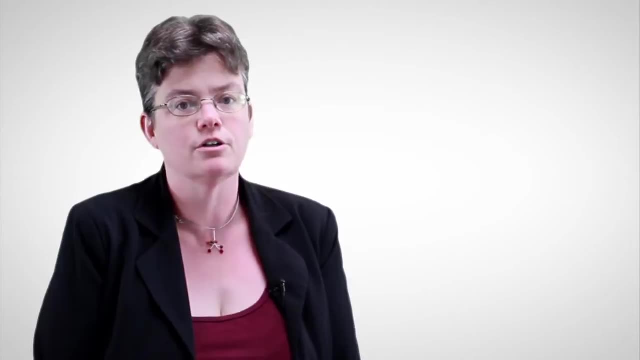 had an absolutely spectacular high school chemistry teacher who got me excited about the chemistry side of things, So when I went to college, I was looking for opportunities to continue to study chemistry. I was very fortunate in my junior year that they hired a theoretical chemist. 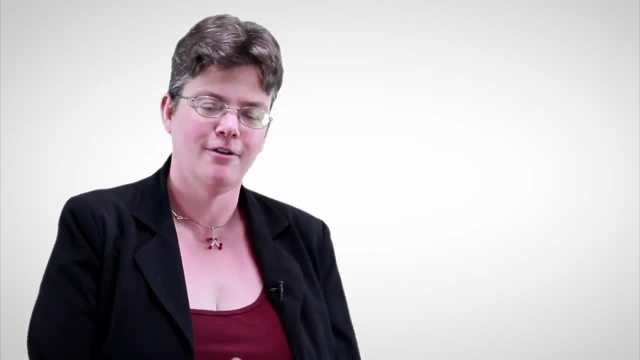 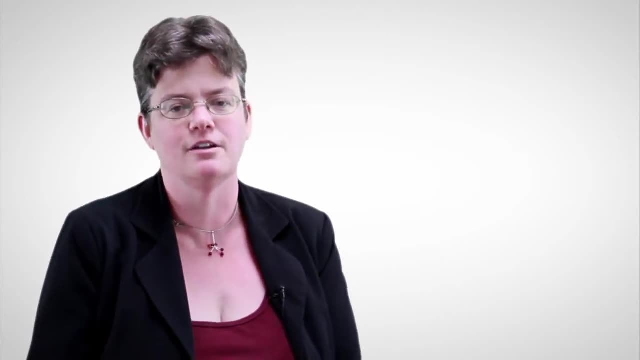 And I realized that that was an opportunity to combine really the pleasure I got from doing the computer programming and understanding ideas through the computers and being able to continue my studies in chemistry, which is what I continued to pursue as a graduate student, postdoc. 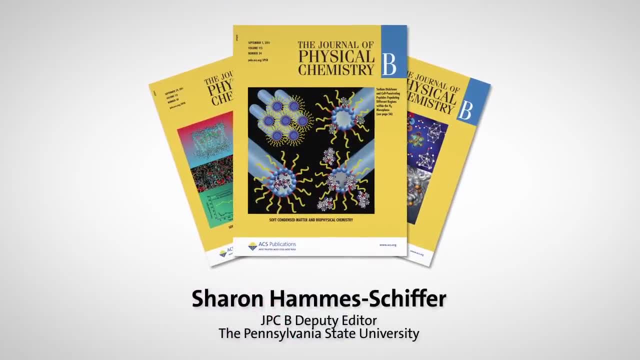 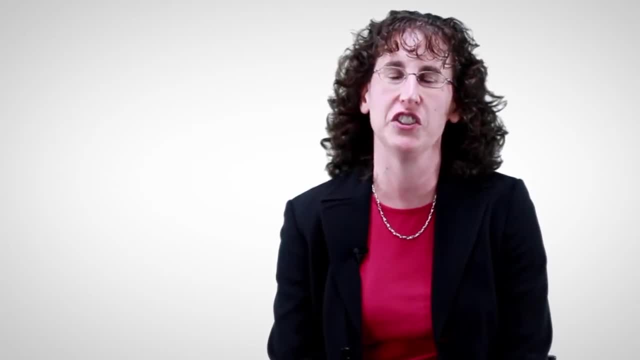 and now in my research at Ohio State. So my father was a professor. He was a professor in chemistry at Cornell And as I grew up, when I was in high school, I told him that I wanted to be anything but a chemistry major. 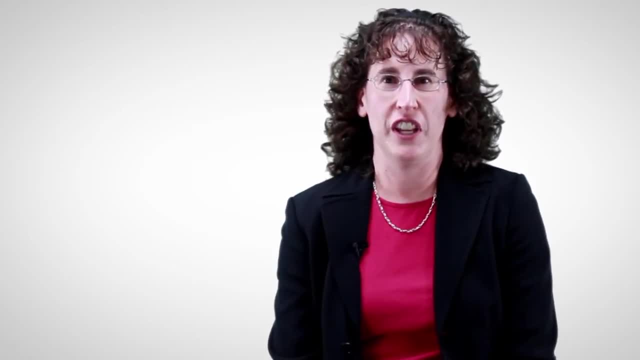 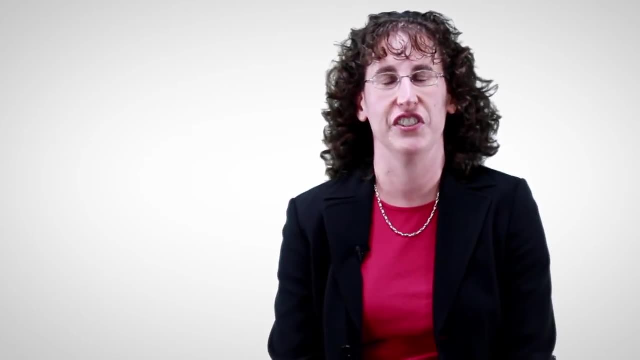 I wanted to be an English major. I loved to read, I loved to write. But then, as I moved toward college, I realized that I really loved math and science And when I got to college, I was trying to choose between chemistry and physics. 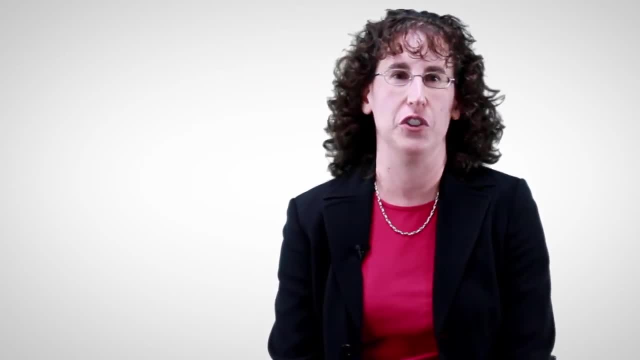 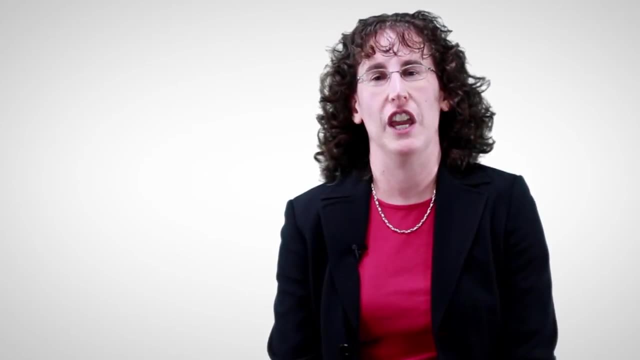 And I realized that physical chemistry was a way I could combine my love of math, chemistry and physics and computer programming as well. Then, when I went to graduate school, I thought I wanted to be a biophysical chemist, so I joined an experimental biophysics group.